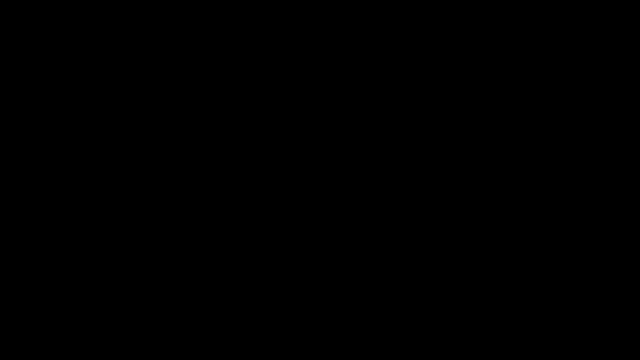 In this video, we're going to talk about how to tell if a graph represents a function using the vertical line test. So let's start with a linear function. y equals x And this function looks like this. It's basically a straight line. 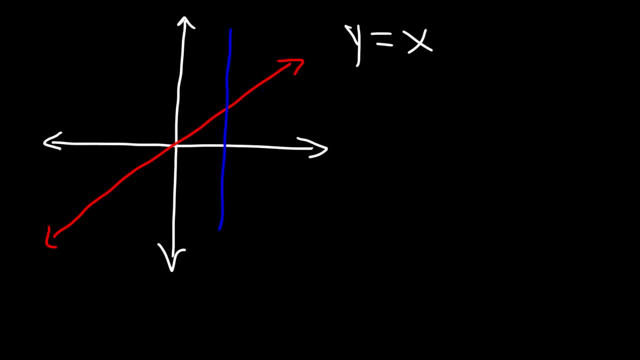 So now what we need to do is draw a vertical line. Notice that the function touches the vertical line only at one point. So that means this graph is a function. Now let's try another example. So this graph is associated with the equation: x is equal to y squared. 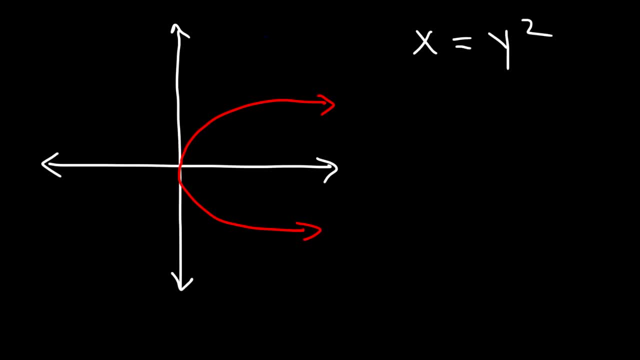 Is it a function? Now, if we draw a vertical line, notice that it touches the line more than one point. It touches that Two points. So therefore, this is not a function. It doesn't pass the vertical line test. Now here's another example for you. 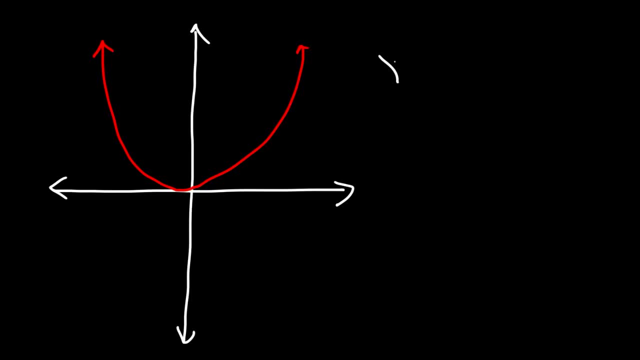 So let's say, if we have a parabola, This is: y is equal to x squared. Is it a function? What would you say? Well, let's see if it passes the vertical line test. Notice that it touched it only at one point. 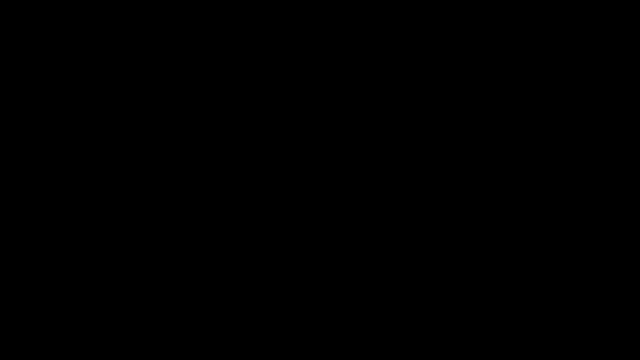 So this passes the vertical line test. Now what if we have a circle? Let's say the equation is: x squared plus y squared is equal to nine. Is it a function? Well, we can clearly see that it's not going to be a function. 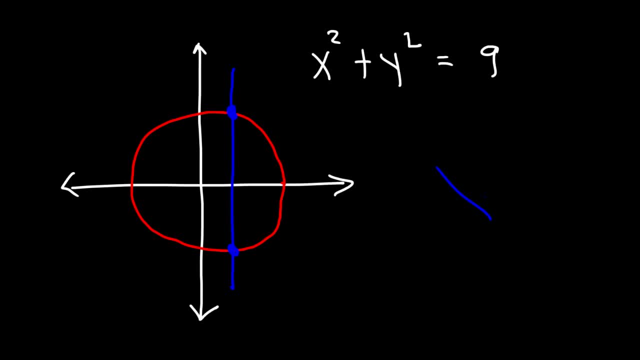 It touches the vertical line at two points. So therefore that's not a function. Now what about this equation? y equals three. Does it pass the vertical line test? y equals three is a horizontal line, And so if we draw a vertical line, it's going to pass the vertical line test. 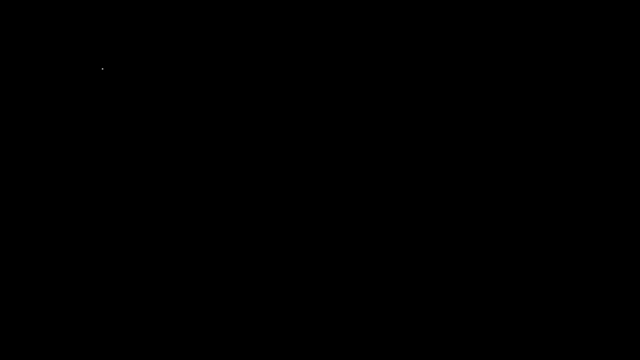 It touched it only. It touched it only at one point. But now what about x equals four? Will that pass the vertical line test? So x equals four is a vertical line, And if you draw a vertical line on it it's going to touch it at an infinite number of. 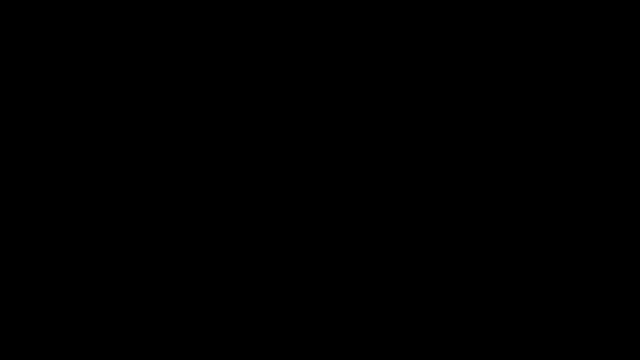 points. So that's not going to be a function. Now, what about these two graphs? Let's say the square root of x And also the square root of x, And also the square root of y And also the absolute value of x. 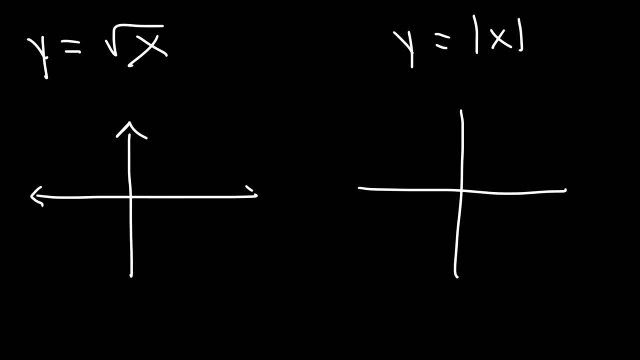 Go ahead and try these two. Determine if they're functions or not. So the square root of x looks like this and the absolute value function is like a v-shape. So this one passes the vertical line test, and so does this one. 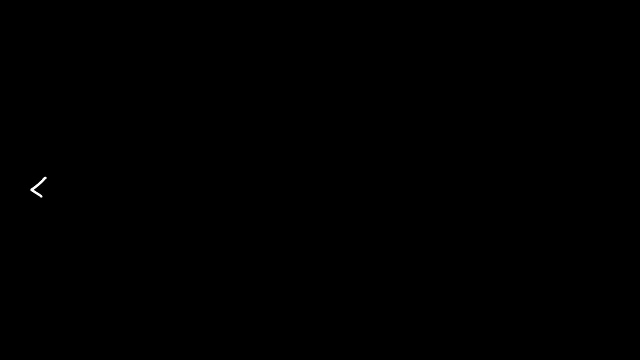 So they both represent functions. Here's another two examples that you could try. Try that one and also this one On the right. this is the graph for sine x. So looking at the first one, we can clearly see that it does not pass the vertical line. 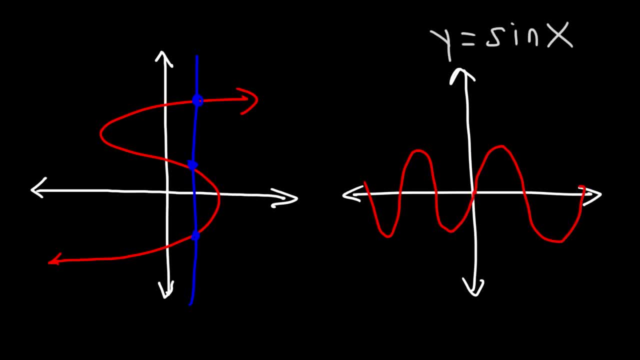 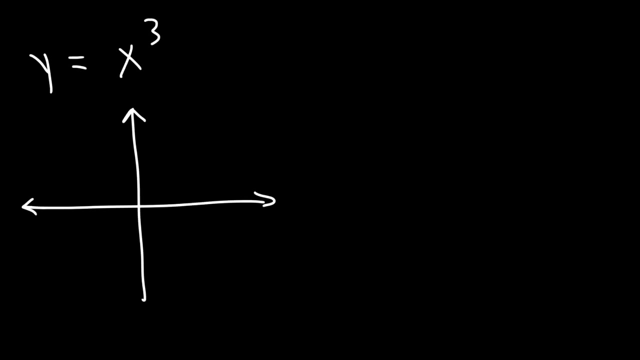 test. Okay, It touches it at least three points for that particular vertical line. Now, the sine function is a function and it passes the vertical line test, but this one does not. Now, what about this function? X, cubed and also the cube root of x. 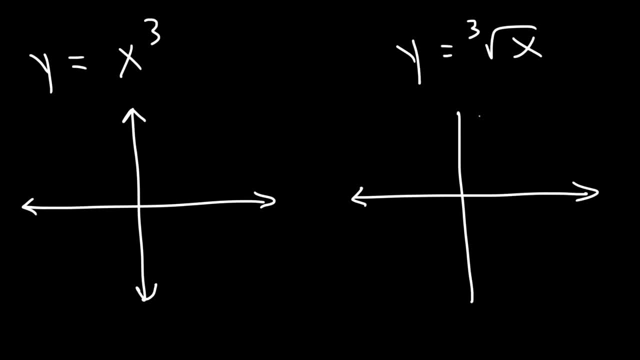 Now the fact that I call it a function And it can't be a function. It can't be a function. It indicates that it's probably going to pass the vertical line test. So x cubed looks like this and the cube root of x looks like that. 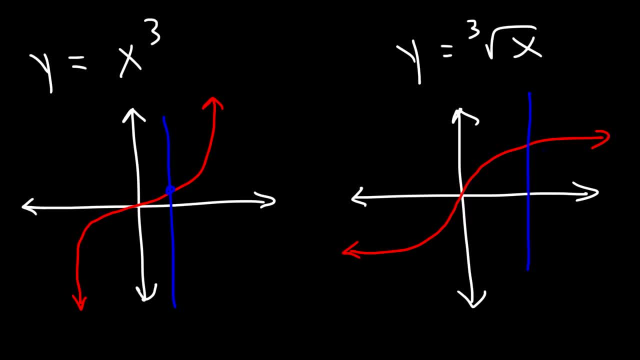 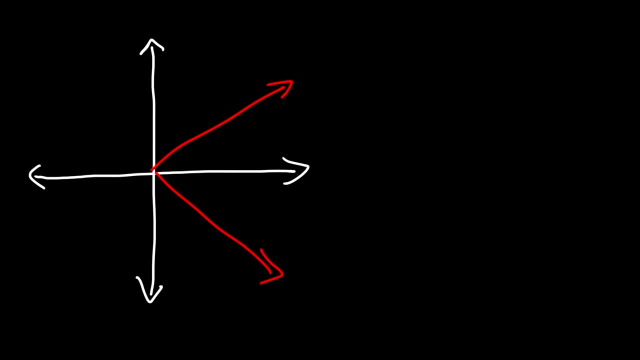 And both of them are functions. As you can see, they pass the vertical line test. And let's consider one more example. So is this graph a function? Well, we can see that it does not pass the vertical line test. It touches it at two points. 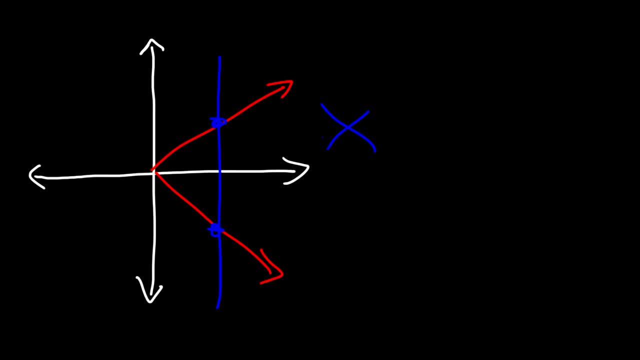 So now you know how to tell if a function or if a graph represents a function using the vertical line test. So if x cubed answers y, that means x is a function. So what kind of function is x? It depends. Sometimes you get a function that says y equals n And sometimes it doesn't. You get a function that says x equals k. That's the one that's going to pass the vertical line test and that's the one that's going to pass the vertical line test. 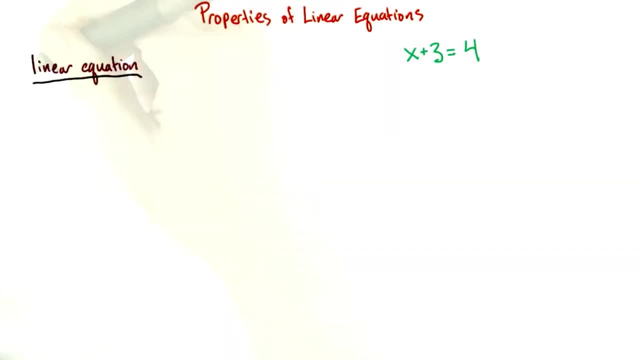 This equation is a linear equation. Linear equations have the following properties: Linear equations must have an equal sign, So here we have an equal sign. Linear equations must have an expression on both sides of the equal sign, And we see here that we have expressions on both sides of the equal sign. And 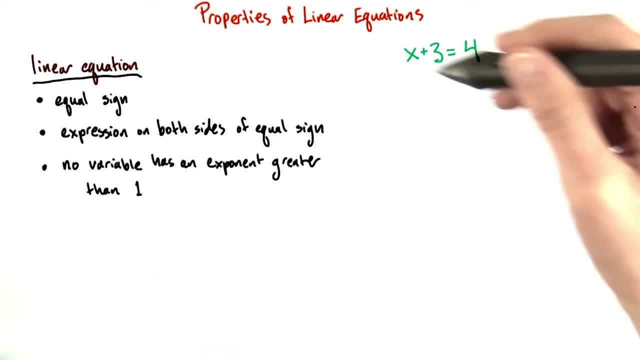 no variables will have an exponent greater than 1. And x here doesn't have an exponent greater than 1.. Previously we talked about algebraic expressions. Algebraic expressions do not have an equal sign. You could only find a value for an algebraic expression if you were given values to substitute in for. 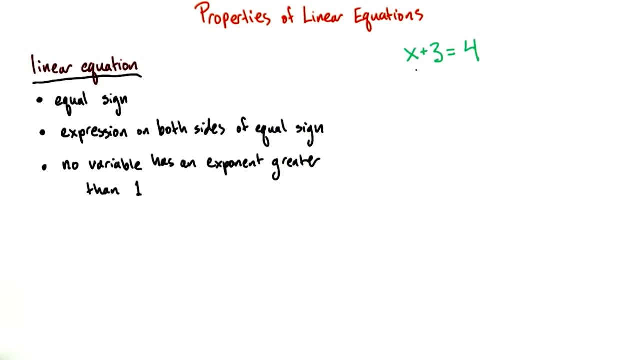 the variables. This is called evaluating an expression. Notice that value is in the word evaluating. This is different from an equation which has an equal sign. When you see an equal sign, you know you can solve the linear equation to find the value for the variable. 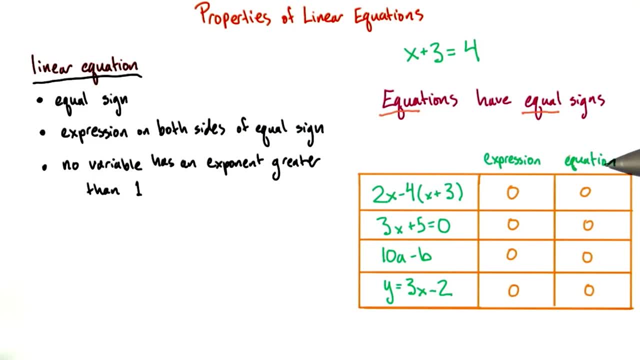 Please indicate if each of these is an expression or an equation. 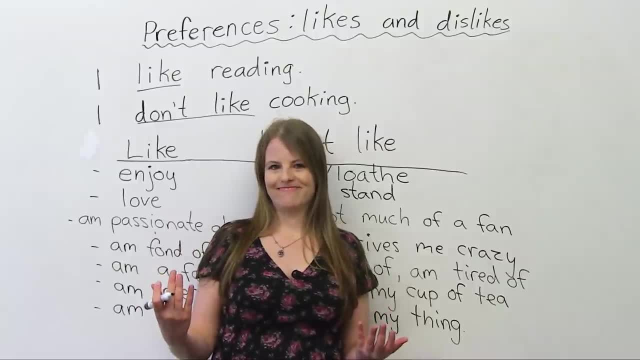 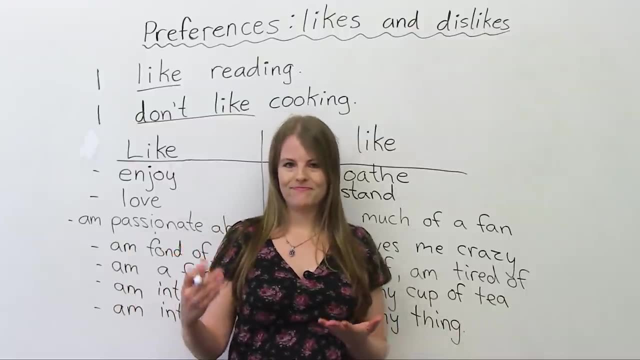 I don't like movies. It gets a little bit boring. Okay, It's, If you're always using this word, there's no problem with the word like, but it does get a little bit boring. So today I'm going to teach you some new expressions that are more exciting, that mean: 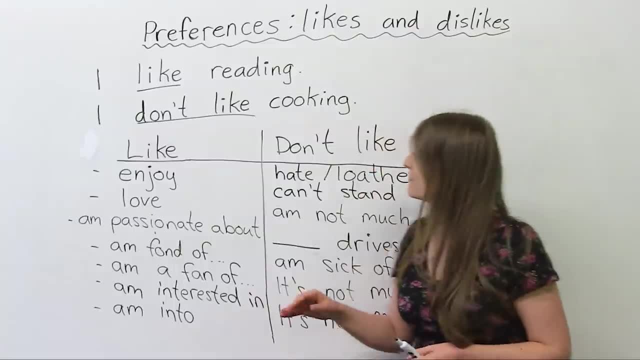 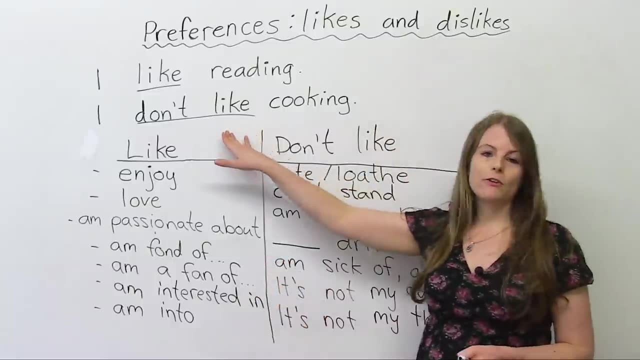 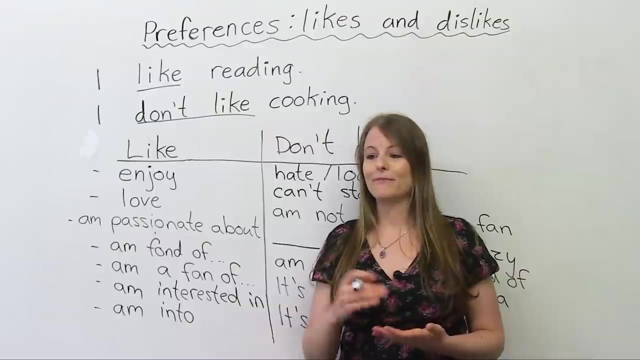 the same thing, So let's look at some of these words. Okay, So I have here the word I like reading. This is something I love doing. And then I wrote something I don't like. I don't like cooking. I'm terrible at cooking and it's actually one of the things I really